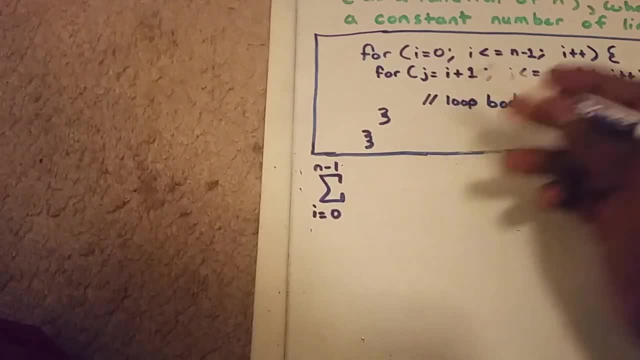 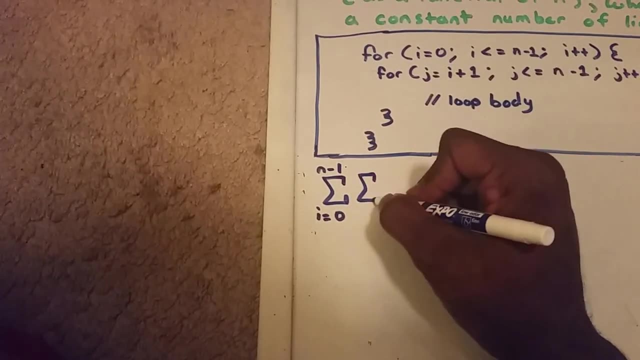 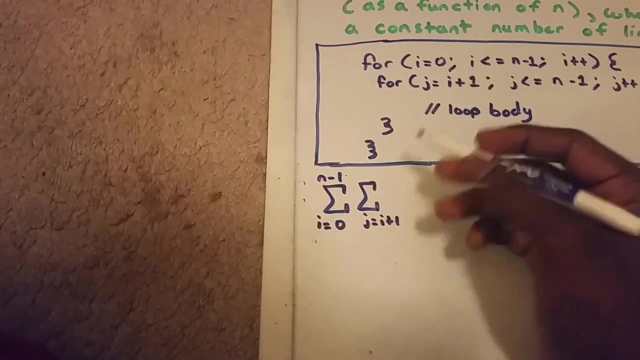 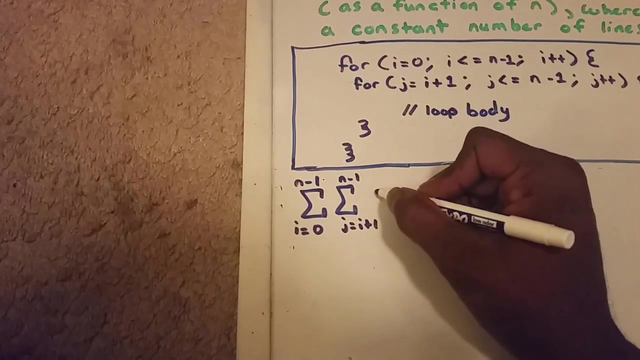 or equal to, so it can go up to n minus 1.. And then we have an inner loop there and it runs from j. so we have an inner loop, let me put that here as a summation- and it runs from: j equals 1 to n minus 1.. So n minus 1.. And inside that we have our so-called 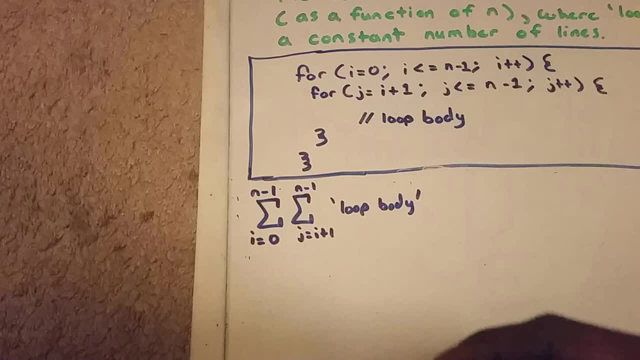 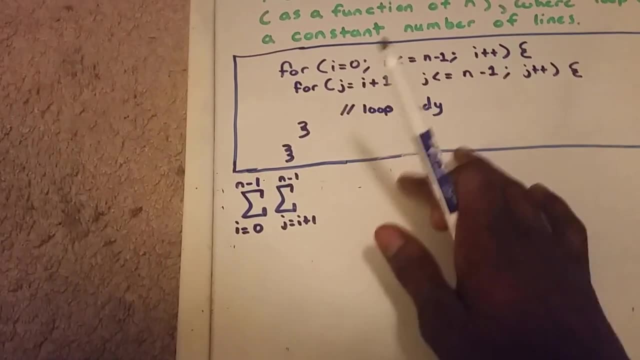 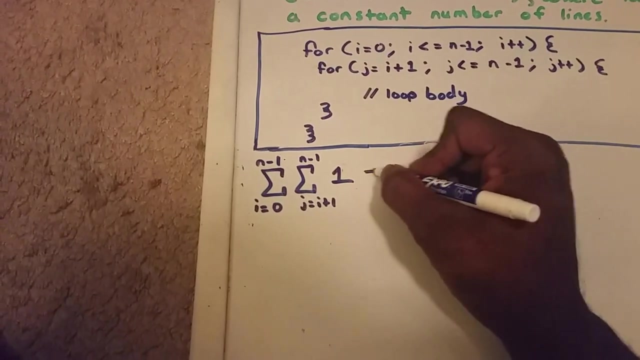 loop body. Now, again, I said a loop body is just a constant number of lines, so we're going to choose a constant for this loop body And the constant I'm going to choose is 1.. Okay, now we want to simplify this because, if we could solve this here, two summations: 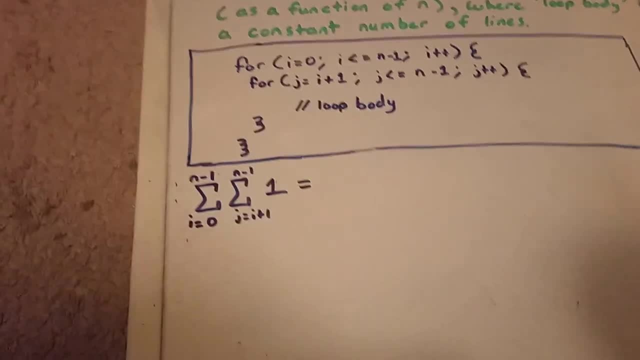 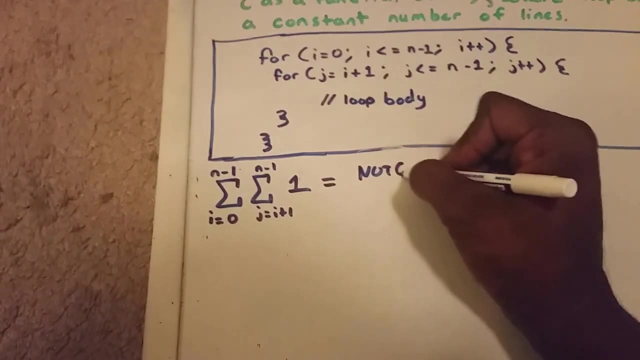 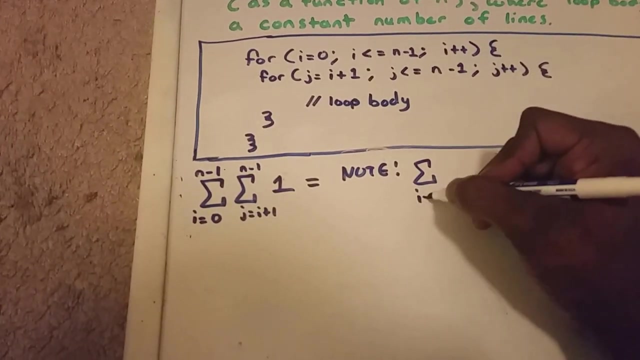 then we can figure out the asymptotic, worst-case complexity. So first I'm going to solve the inner loop, And in order to do that we have to know something. So I'm going to put a note here, So we're going to note that the summation from i equals m, which m is just some constant. 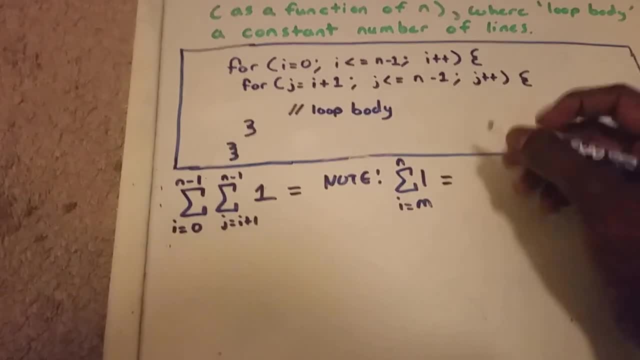 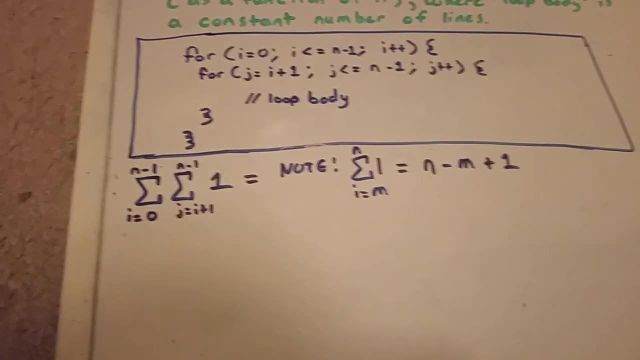 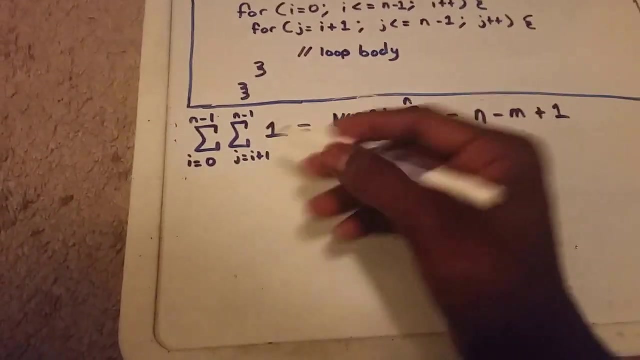 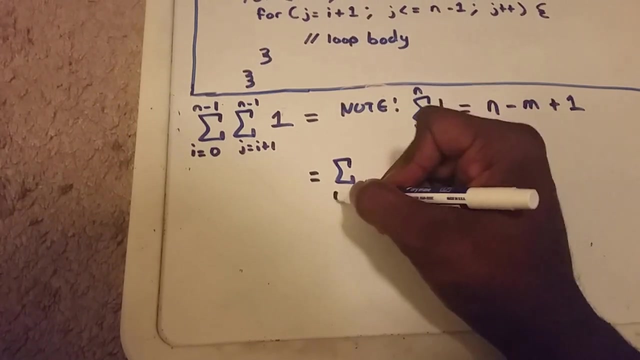 to n of 1 is equal to n minus m. Okay, that's one of the formulas for summations. So now we're going to start writing our equation. First, I'm going to rewrite the outer loop summation, which runs from: i equals 0 to n. 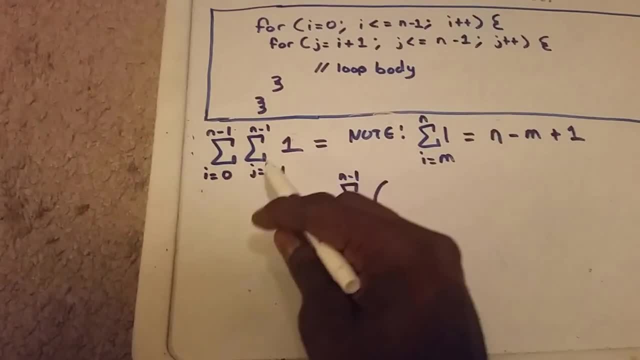 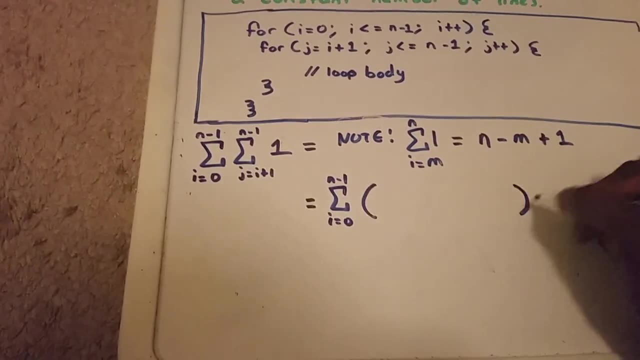 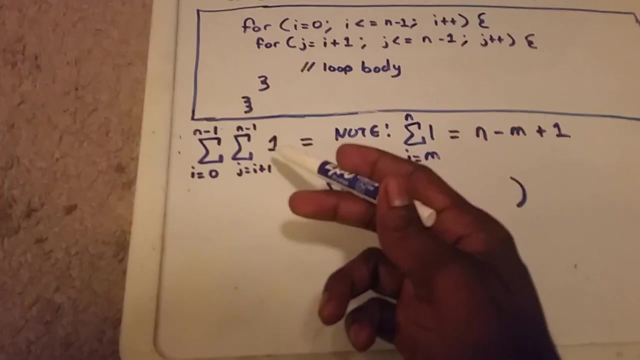 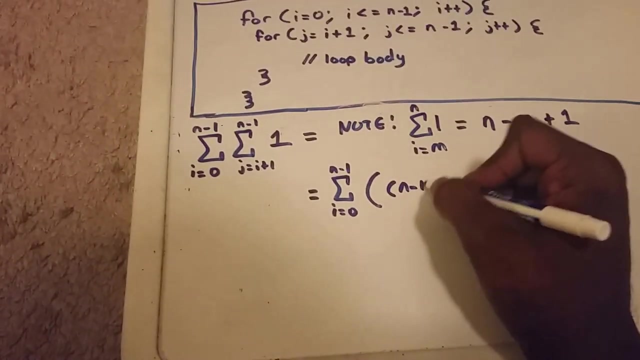 minus 1.. And inside here, that's where our inner loop, or our inner summation in this case, will be. Okay, I'm going to close it here, And now let's try to figure out how this formula relates to this inner solution, inner summation. So our n is equal to n minus 1.. So we have 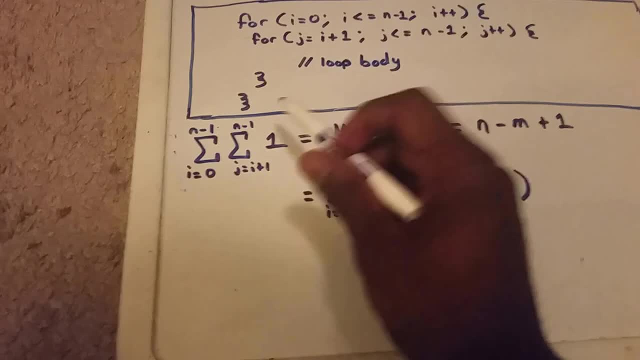 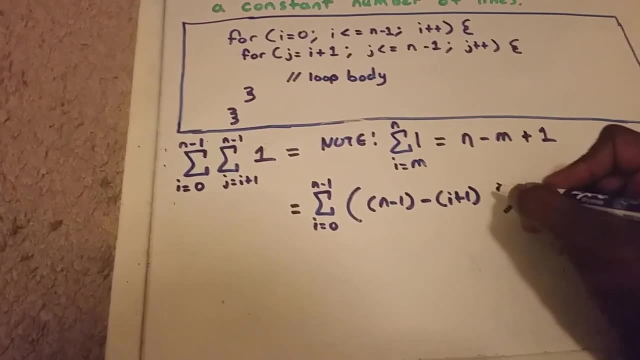 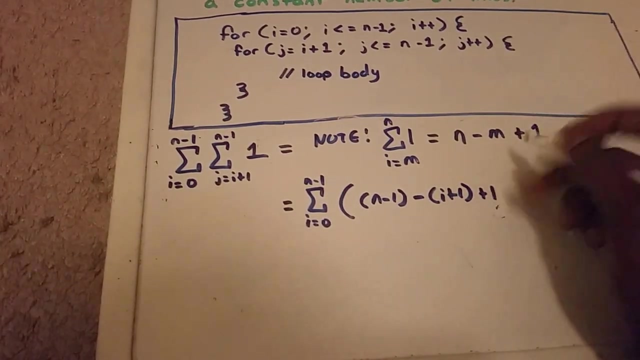 n minus 1, minus our m is i plus 1.. So i plus 1.. And then we have to add in that 1 there, So plus 1.. Then we're going to slightly rewrite that there So you can see it very clearly So. 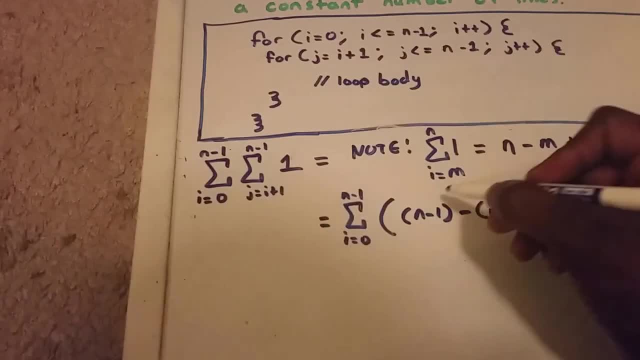 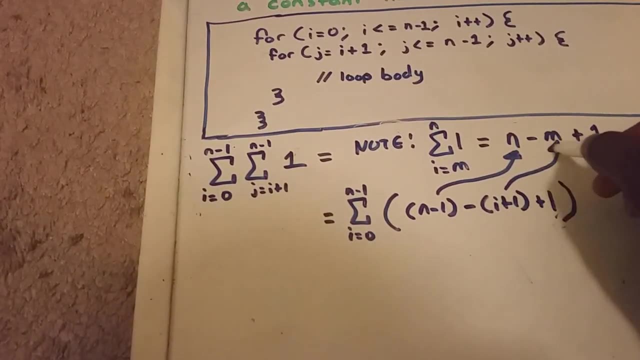 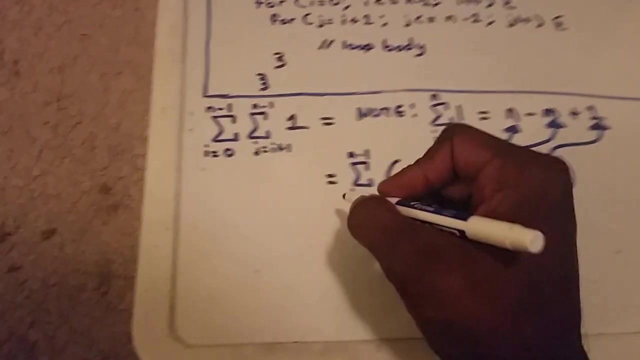 that's a 1 there. Okay, And again, this n minus 1 refers to this n, This i plus 1 refers to the m And the 1 refers to the 1.. Alright, So now we're going to just try to simplify this a little bit more. I'm going 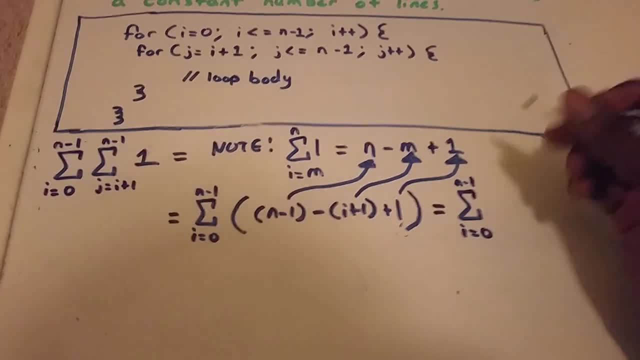 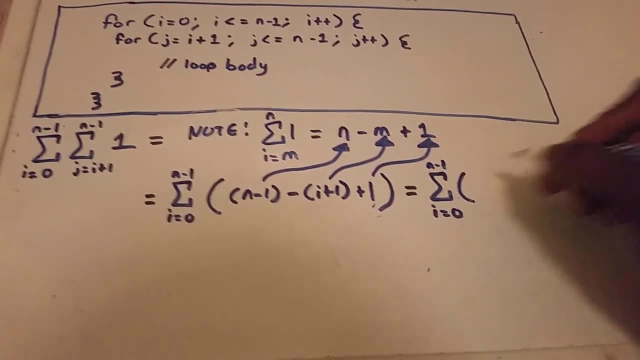 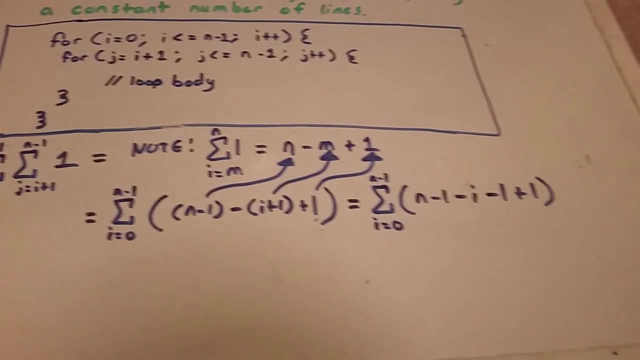 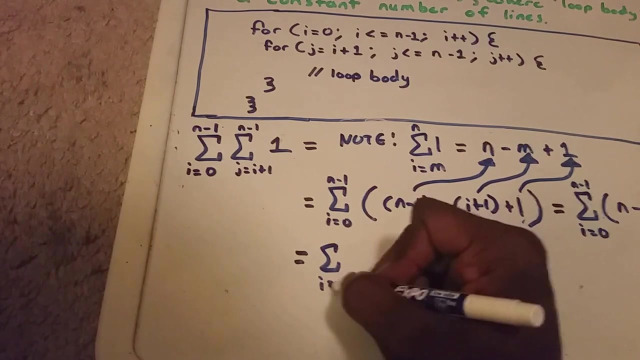 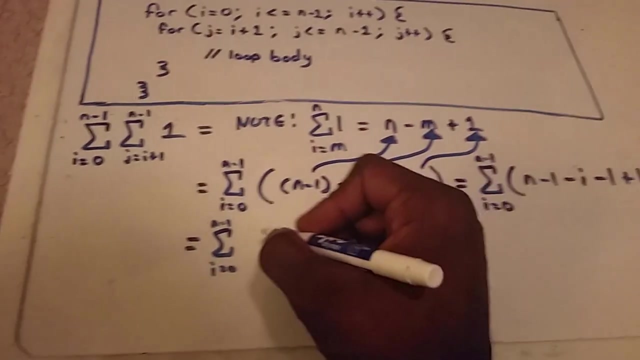 to rewrite the outer summation, loop summation, and we're going to start simplifying within this summation here: n minus 1 minus I minus 1 plus 1, and if we rewrite that again from I equals 0 to n minus 1, we see that the minus 1 and the plus 1 can cancel out. so now we get. 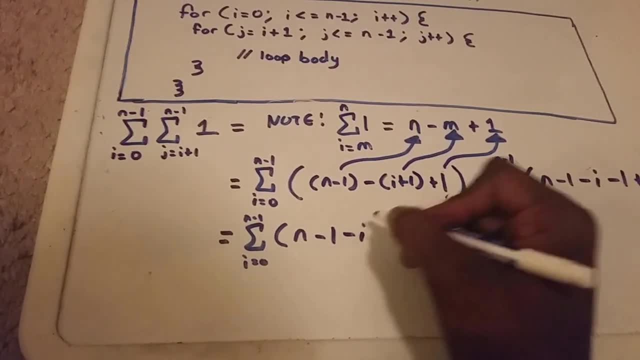 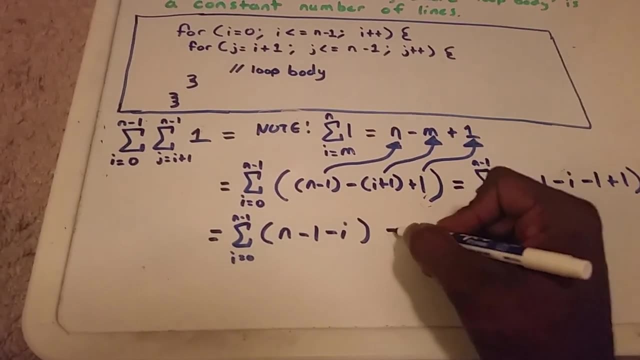 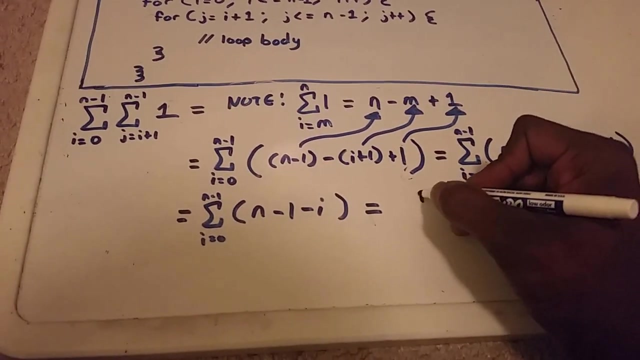 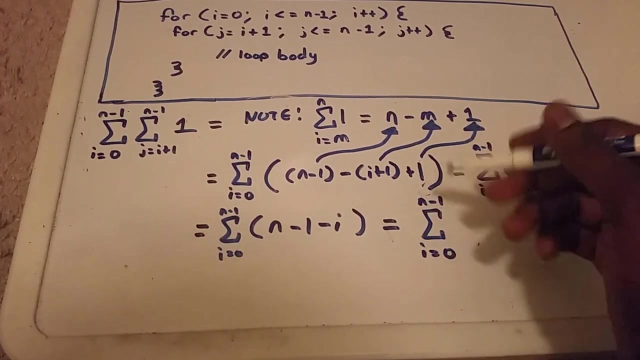 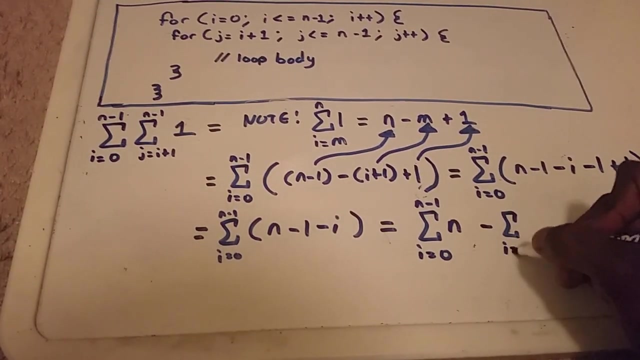 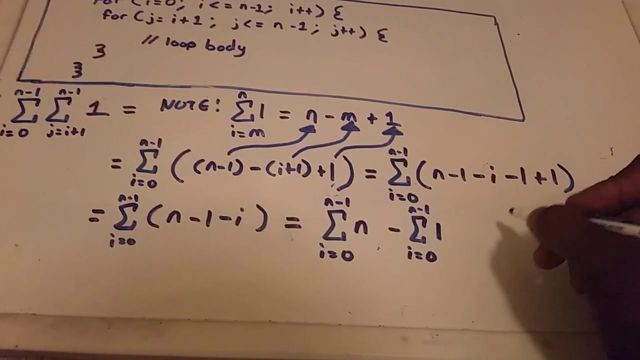 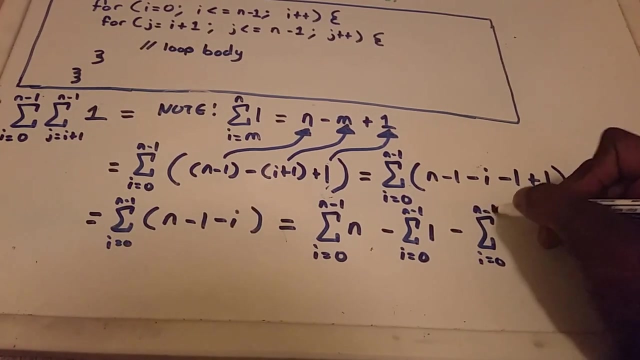 n minus 1 minus I. okay, and now, using the laws of summation, we get to rewrite the equation like so: from I equals 0 to n minus 1 of n minus summation from I equals 0 to n minus 1 of 1 minus the summation from I equals 0 to n minus 1 of I. okay. 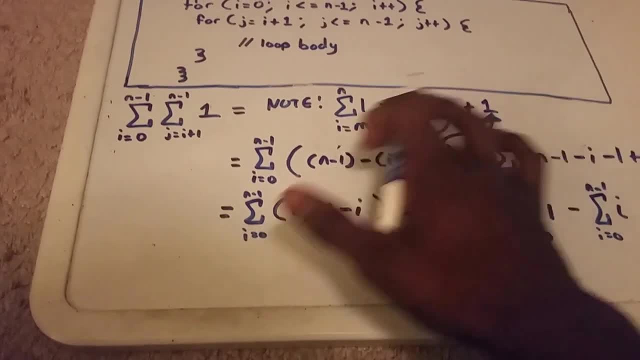 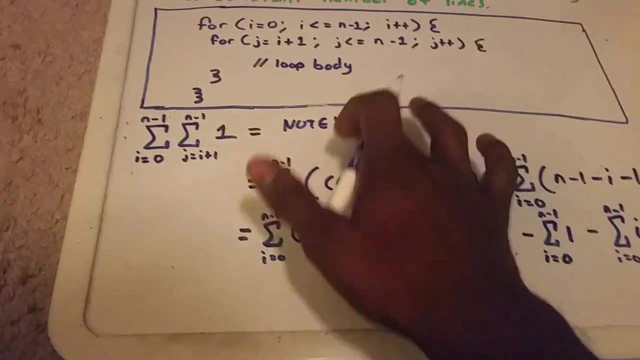 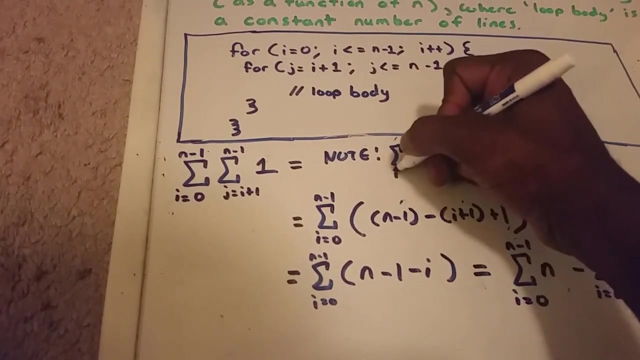 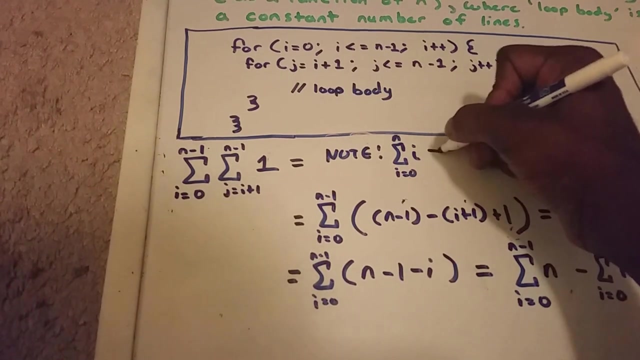 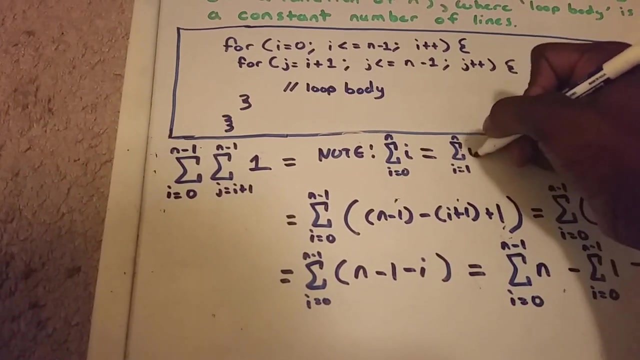 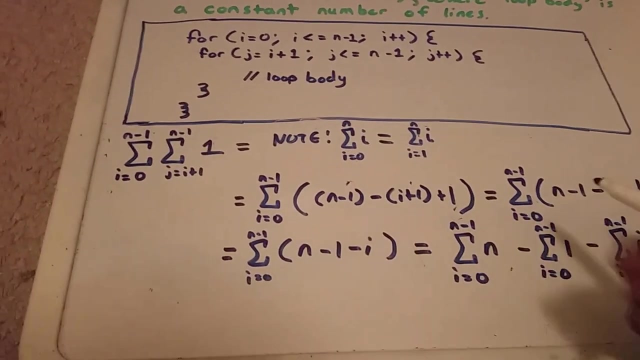 so now another thing to note. I'm going to erase this previous note up here, okay. another thing to notice: that the summation from I equals 0 to n of I is equal to the summation from I equals 1 of n to I. alrighty, so let's rewrite this. 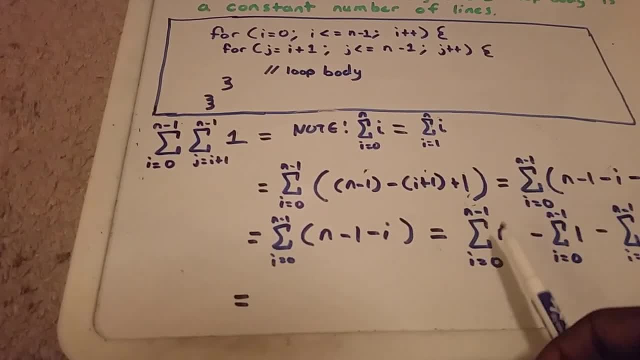 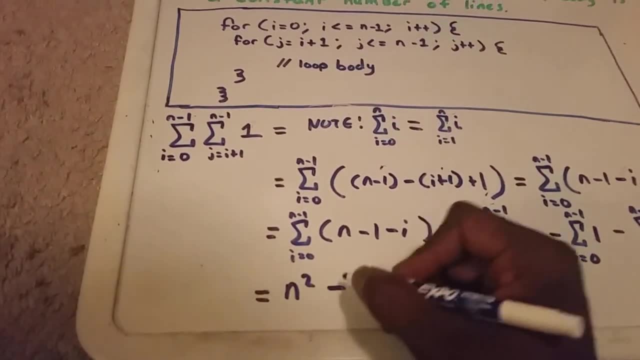 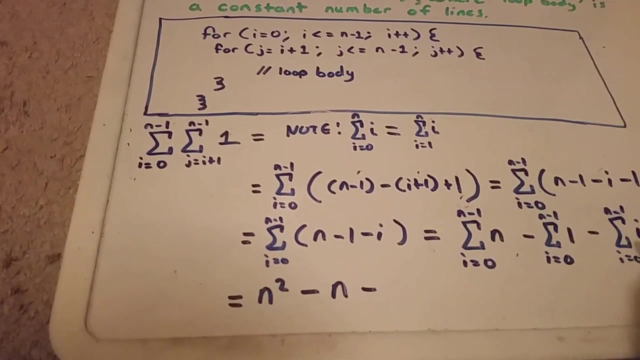 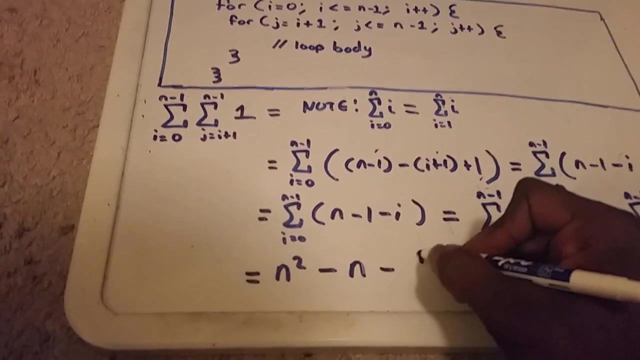 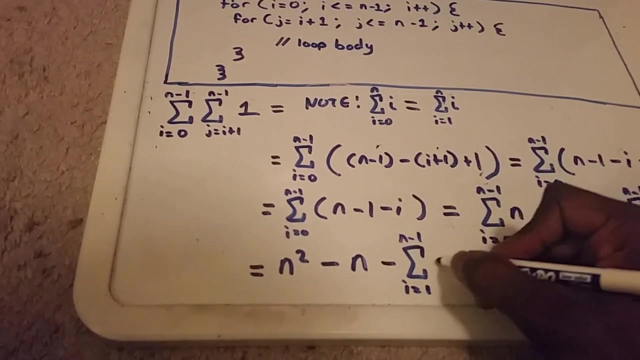 again now. so here we get n times n, so we get n squared minus. we get in here minus. well, we said that this summation is equal to that there, so let's rewrite it like that, I wish: from I equals 1 to n minus 1 of I. and now let's rewrite this: 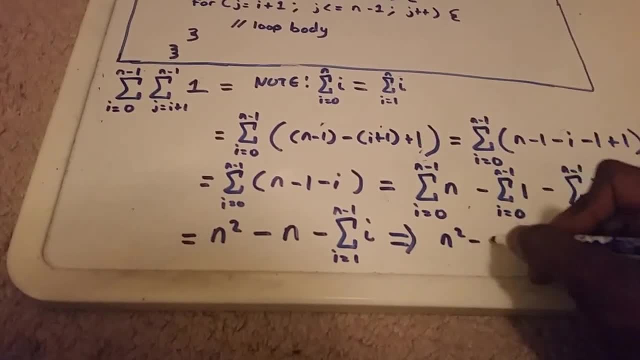 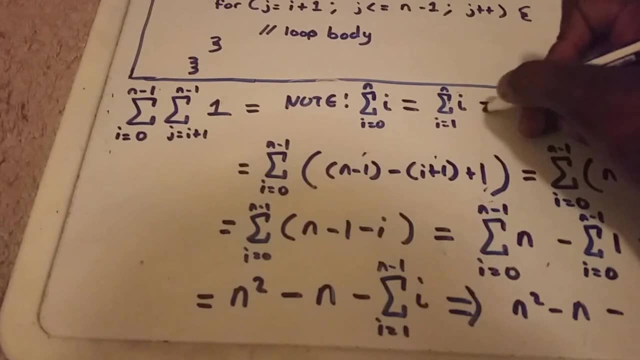 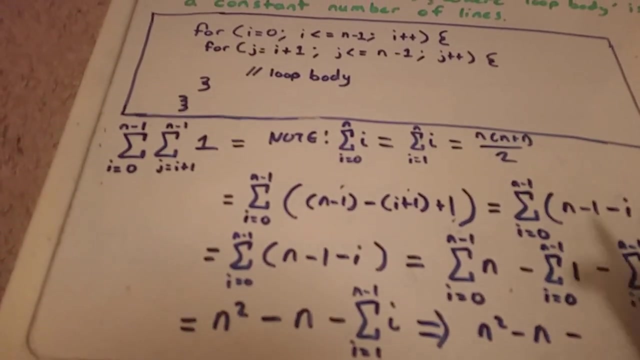 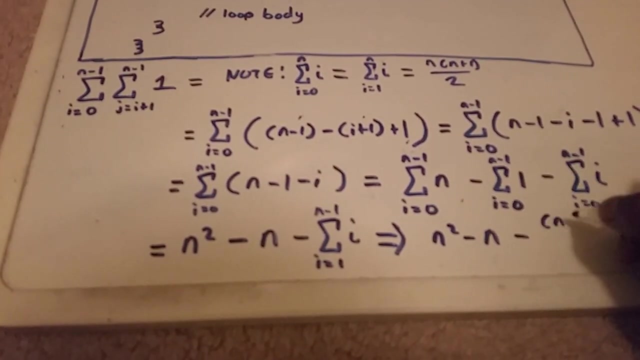 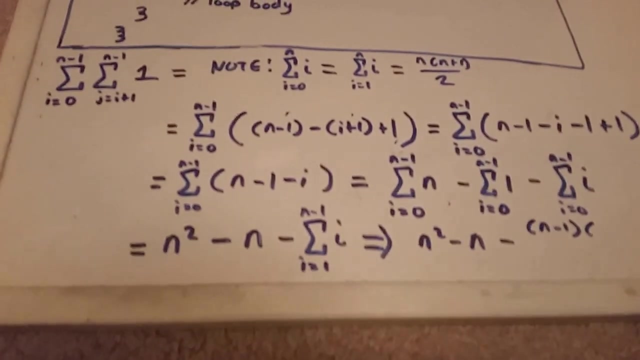 one more time and square it minus n, minus. there's a formula here, for I put that here as well: it's n times n plus 1 divided by 2. so there we go and use that same formula, replace n for n minus 1, and so we get n. 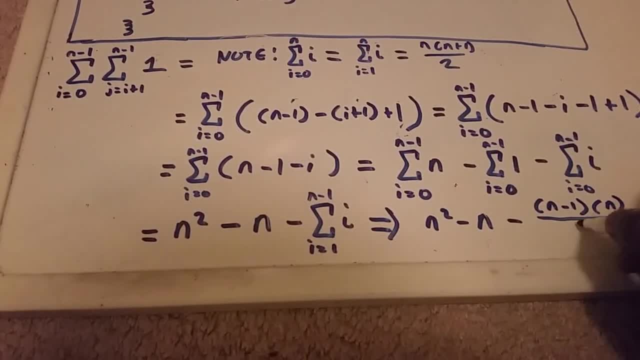 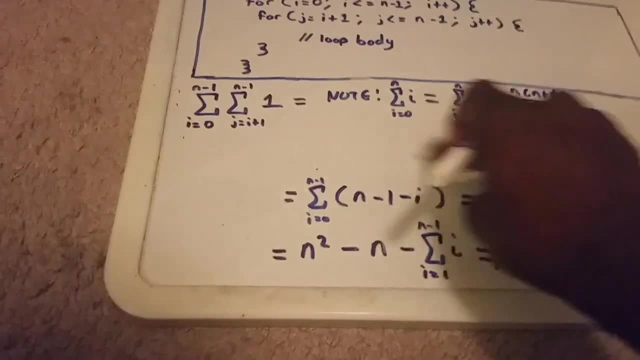 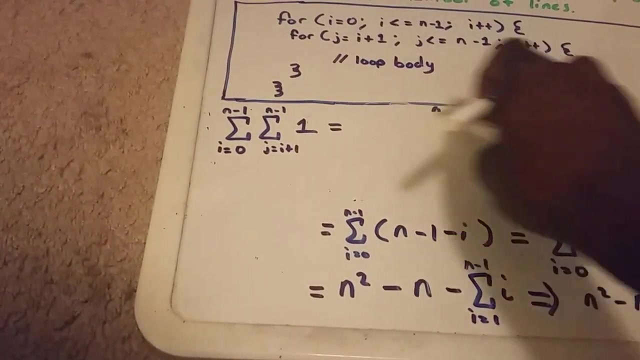 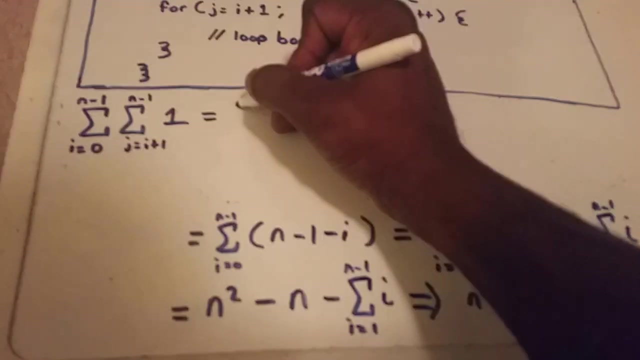 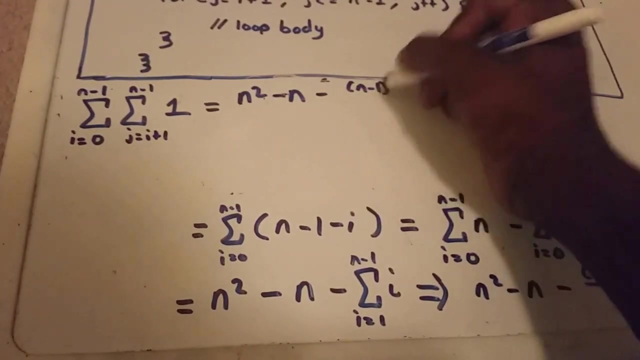 minus 1 times n. 2. alright, looks like I'm running out of space. Gotta start erasing, okay. so we're going to start back from the top here and we're going to read the equation down below. so we have n squared minus n, minus n, minus one times n. 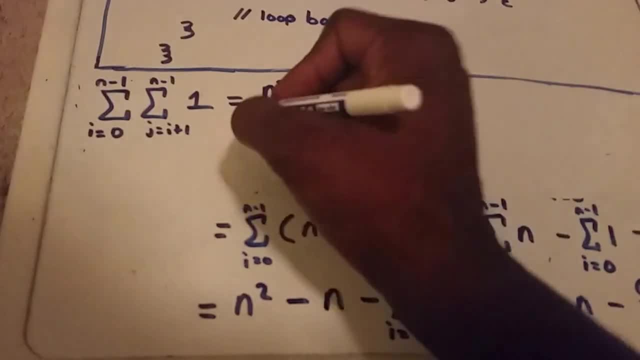 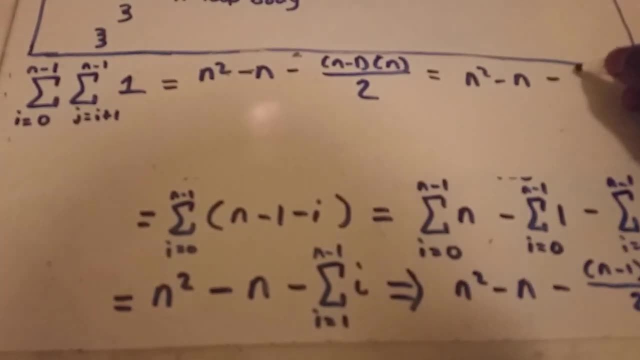 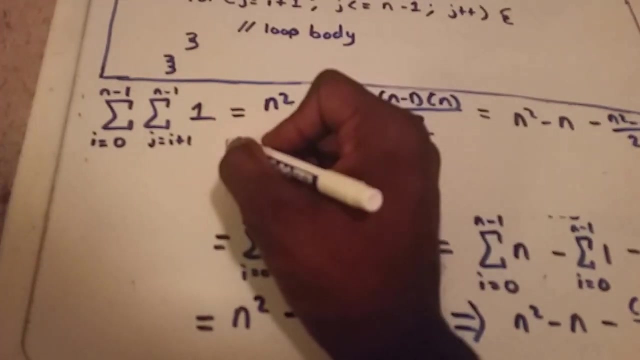 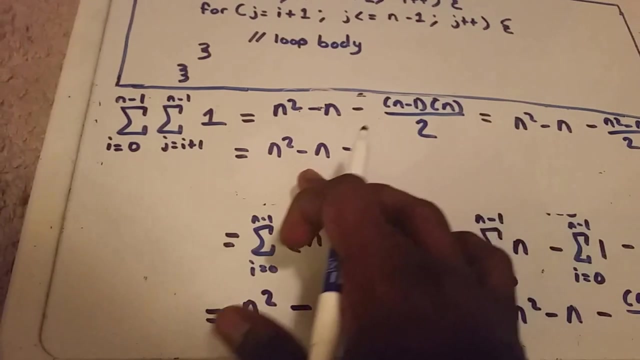 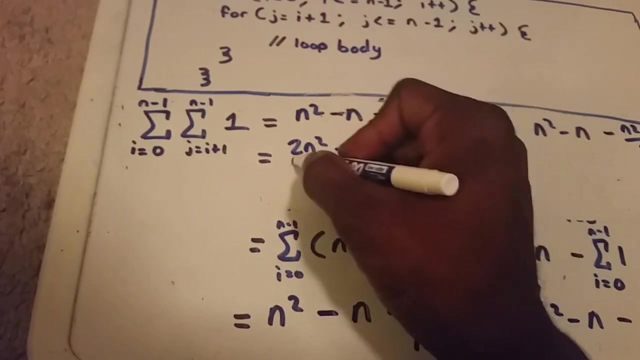 divided by 2. okay, I'll simplify this a little bit more: n squared minus n minus n squared minus n divided by 2. okay, so now we're going to keep simplifying, so we get. we get 2 n squared minus 2. n divided by 2 minus n squared minus n.